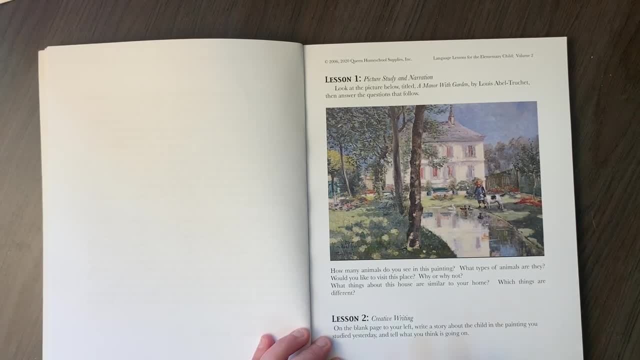 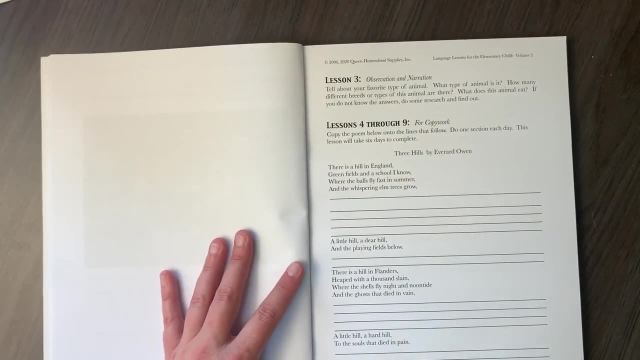 about the picture. and then here we have a creative writing, So tell a story of what you see happening in the picture. and lesson three. So there are 180 lessons. so it's meant to be done once a day, 180 days of the week. We do it a little differently. 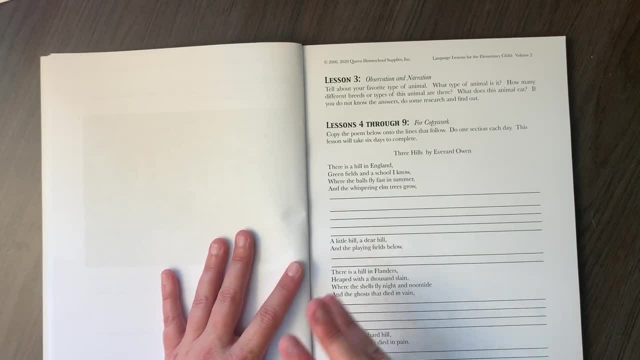 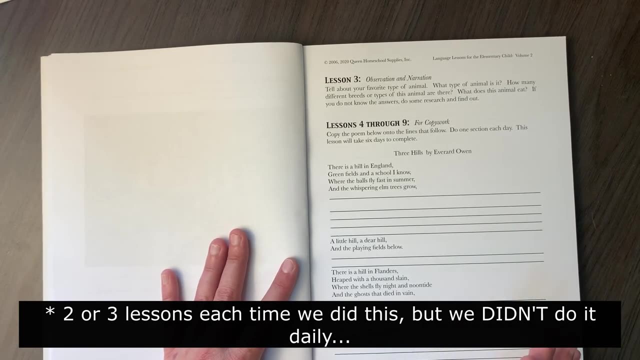 I will generally do. this year I was doing two or three lessons depending on the child and this coming year I plan on doing one or two lessons depending on the lesson, because we do do a lot of other language arts and I think once we finish that one, I feel like we can take this one. 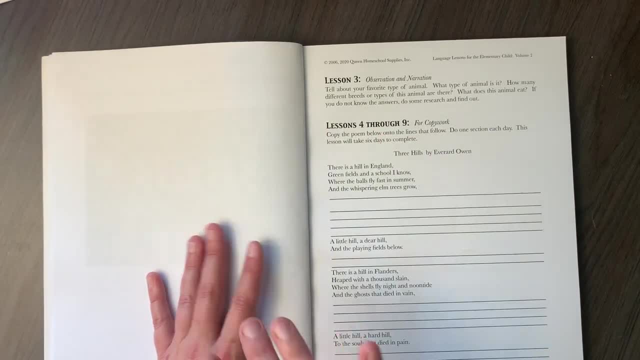 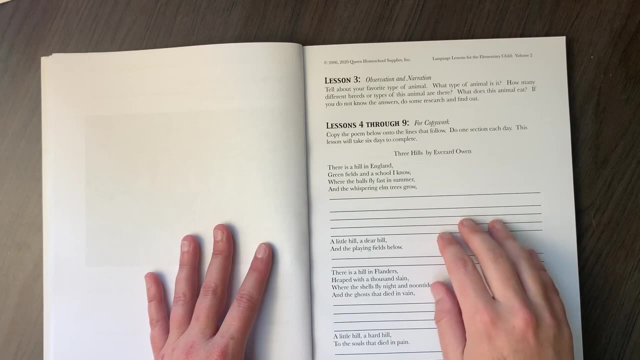 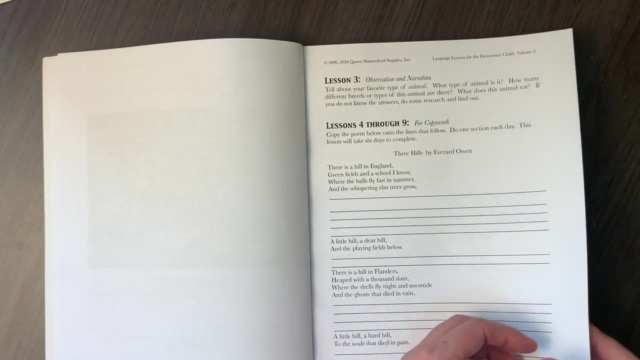 a little more slowly, All right. so lesson three, observation and narration, talking about a favorite type of animal. Lessons four through nine is just some copy work. so very, Charlotte Mason. so they're copying. So this is one lesson, Another lesson. so this is each one lesson here. so lessons one through four through nine, My kids- 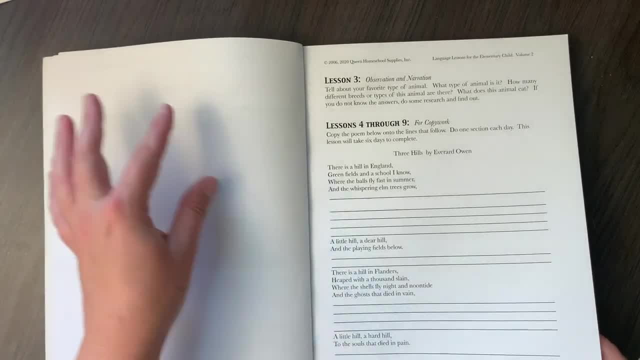 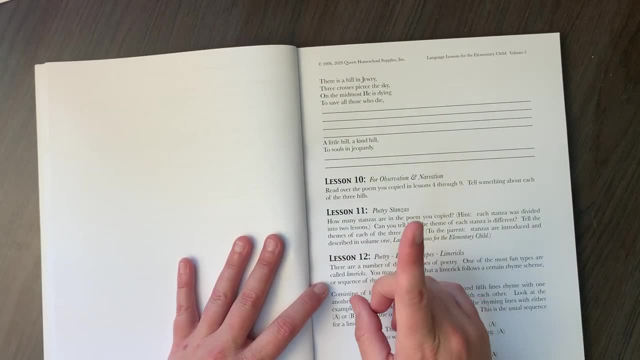 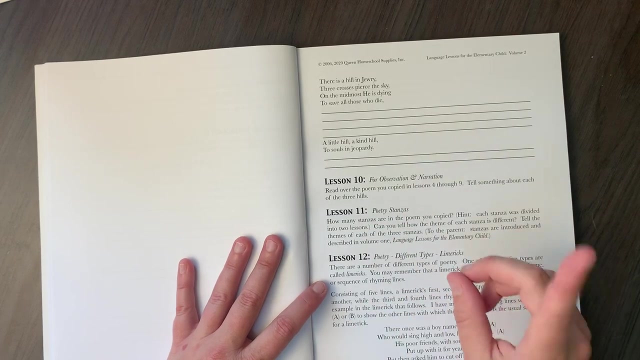 don't love writing, so that's when I would assign one lesson versus two lessons. if it was something else, All right, so copy work till there. I will say one of my complaints, one of my complaints about these books is they don't give enough space for my one of my children. He writes pretty large. 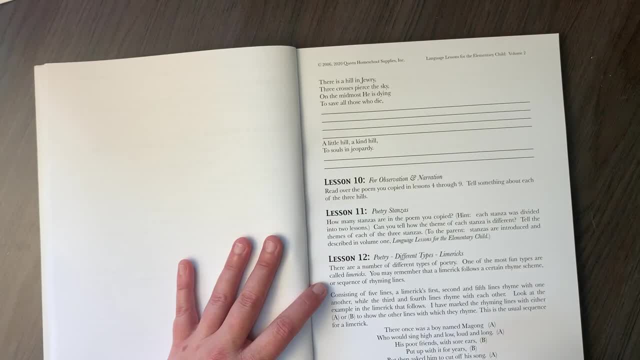 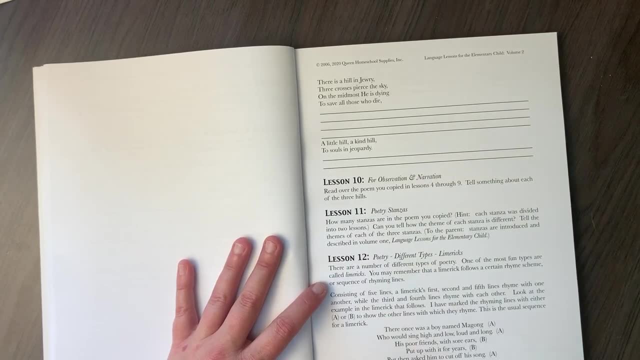 but not crazy large, and he often does not have enough space to write. So that is one one issue that I have found with these books. but he's managing. He does need to learn how to write a little smaller, but it would be nice if we had a few extra lines for each of. 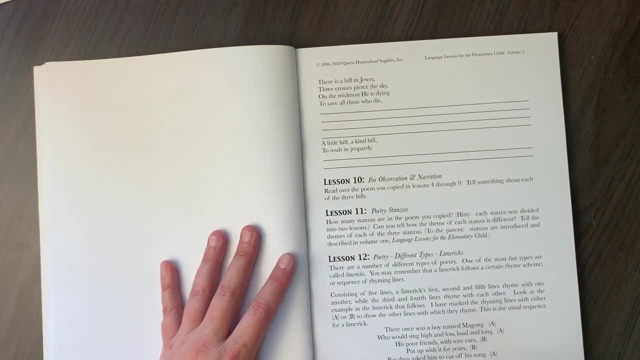 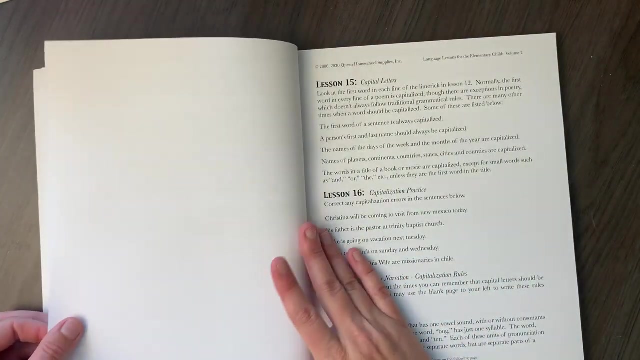 these All right. so lesson 10: read over the poem, tell about each of the three hills. We have stanzas, so poetry stanzas, talking about poetry. and then they're going to be doing some limericks, so learning about limericks. So there's a few lessons on that and then you get into the grammar. 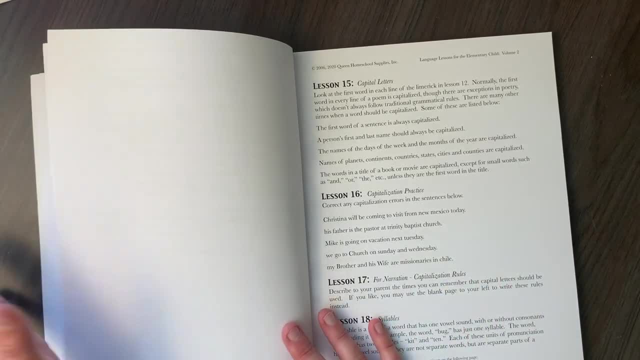 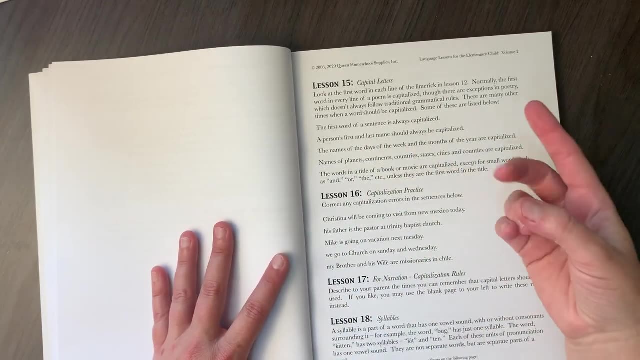 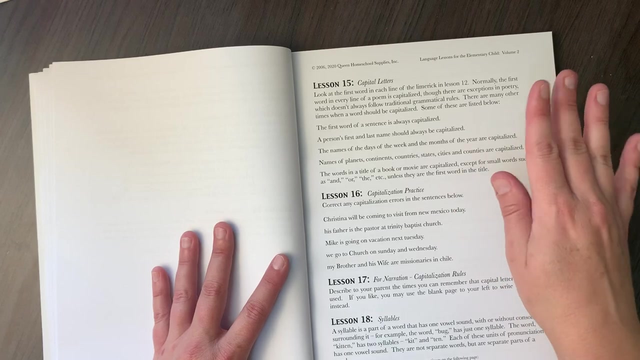 So it just kind of rotates between picture study, poetry, talking about poetry, observation, and then we have grammar days, which I usually do two lessons at a time, because sometimes they only have explaining one day and then you start doing something the next day, So there's capital letters. 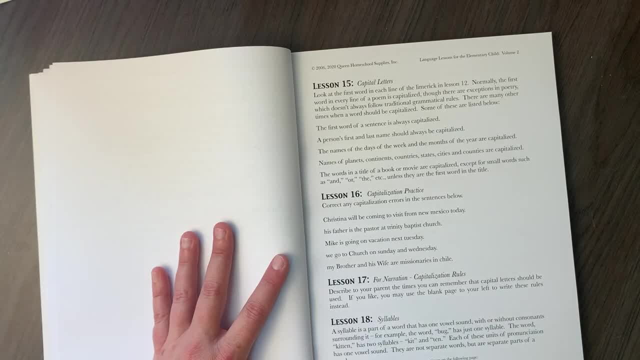 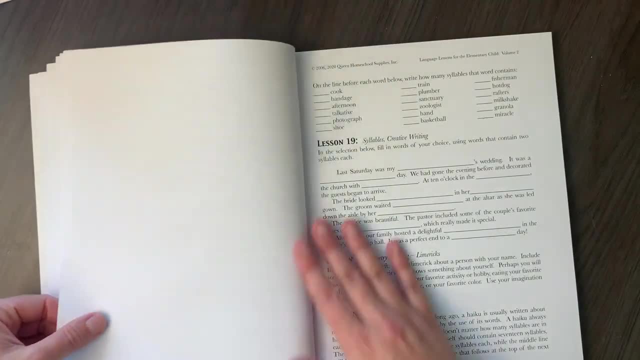 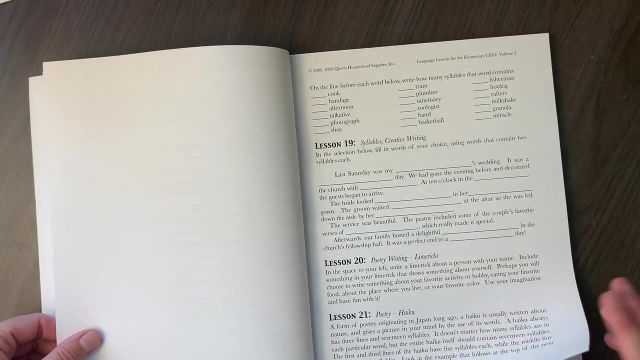 capitalization practice for narration, capitalization rules. so talking to a parent about it. syllabus, syllables, so learning about syllables. so a lot of this is a review from last year. they just kind of build upon what they did last year. Now we're talking about limericks again and the haiku, so they learn about. 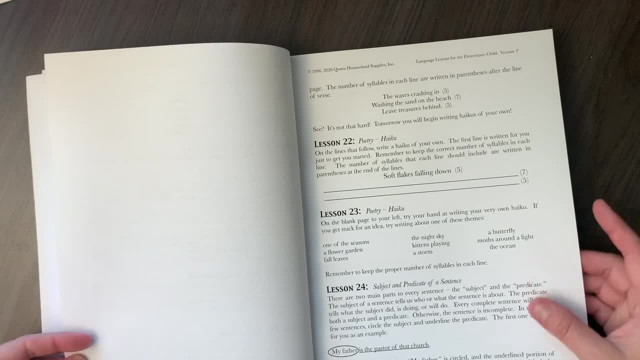 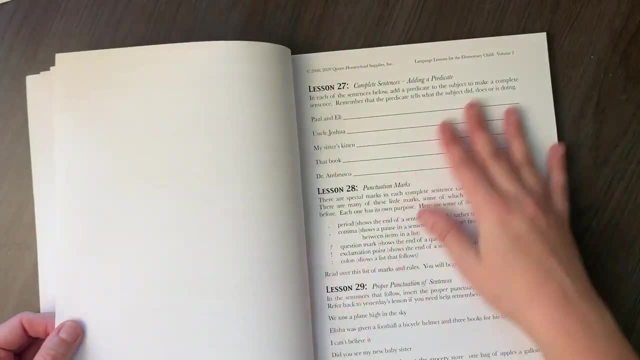 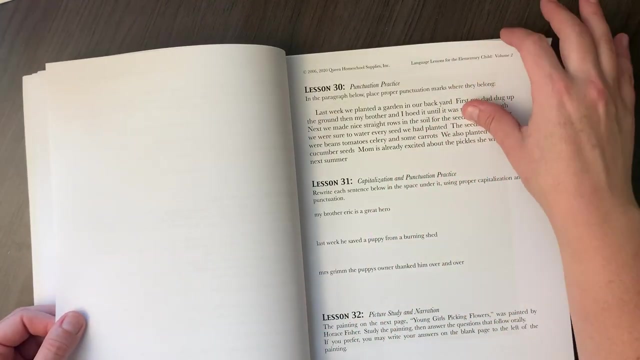 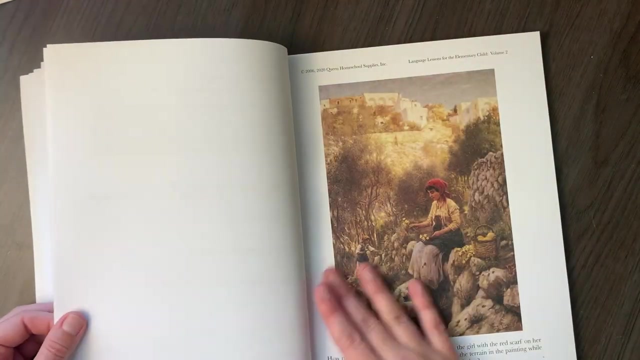 the haiku, so there's more about the haiku. and then we have subject and predicate of the sentence, complete and incomplete sentences, adding subjects, complete sentences, punctuation marks, proper punctuation of sentences, punctuation practice, capitalization, punctuation practice, picture study and narration, and then that is part of this new section here and 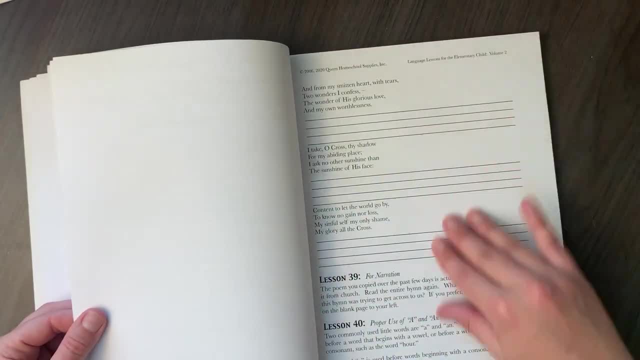 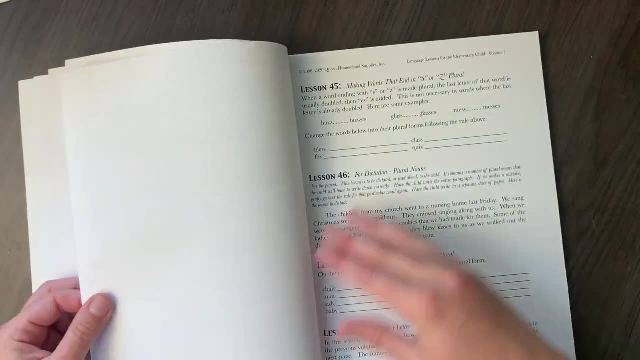 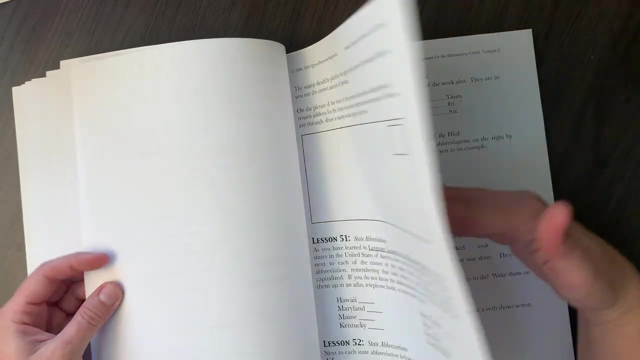 then each section is very similar. we'll go through some copy work, we'll do narration, we'll learn about grammar rules, and then they usually talk about some form of writing. so here's writing a letter, and last time it was poetry, right. so we have writing a letter addressing the envelope. 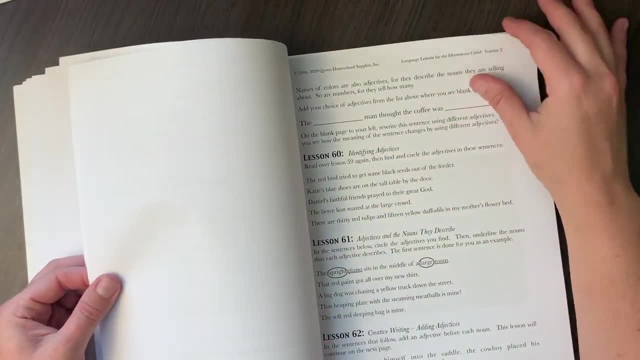 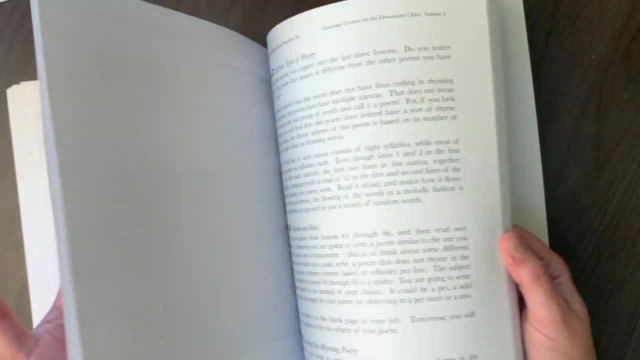 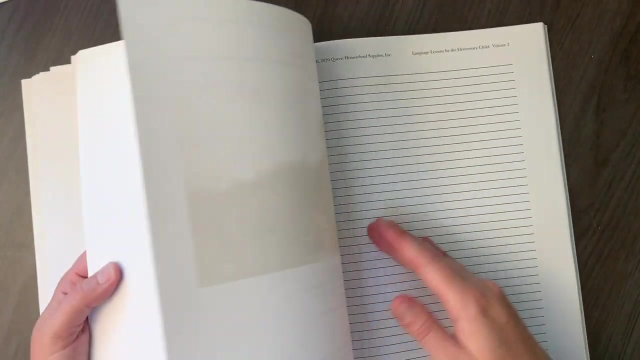 abbreviations, so very kind of natural way to move from one thing to the other, and I would just say there's some breaks in the middle and you just kind of go through that pattern of narration. copy work- oh, what's this? looks like creative writing. so you're writing a story, more copy work. 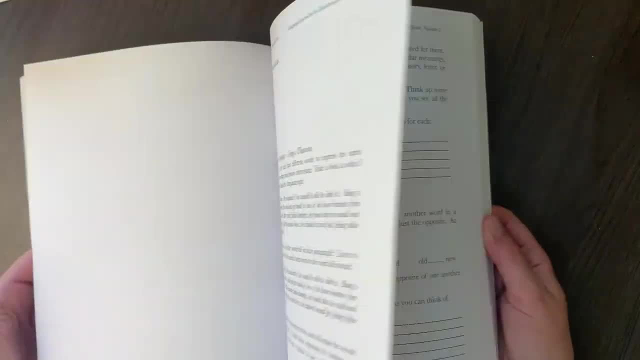 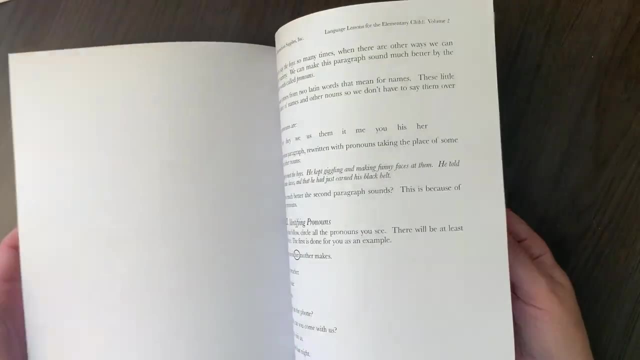 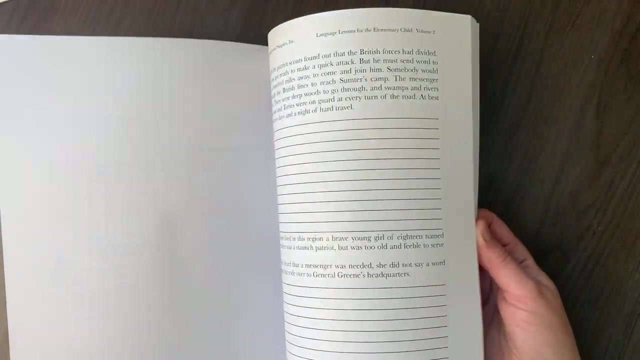 yeah, and then we'll get into the grammar. so just a predictable kind of pattern. but you just cover everything a little bit in more in depth, each, each book, I would say, and towards the end they do start to review the concepts that they learned. so we'll have the copy work. much bigger passages as 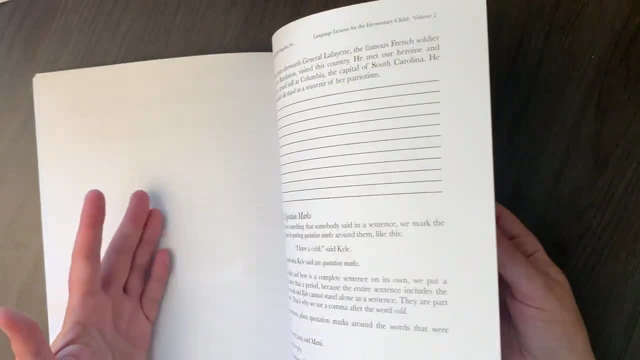 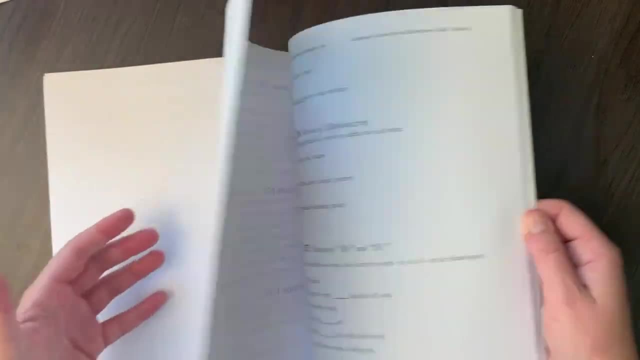 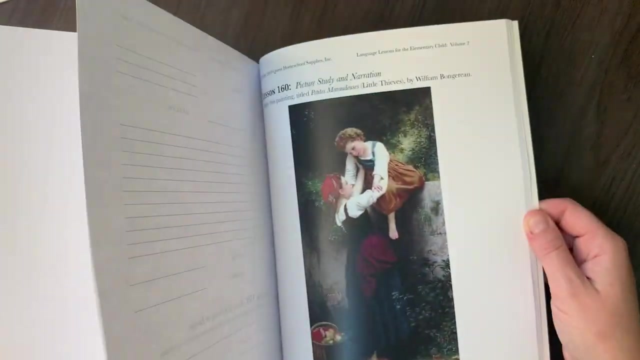 you can see, towards the end here we have quotation marks and then review. so review of using and and review of punctuation marks, review of contractions, review of elf- elf alphabetizing it's an, it's letter writing, writing another letter and then more the same, yeah, so, like I said, we have really